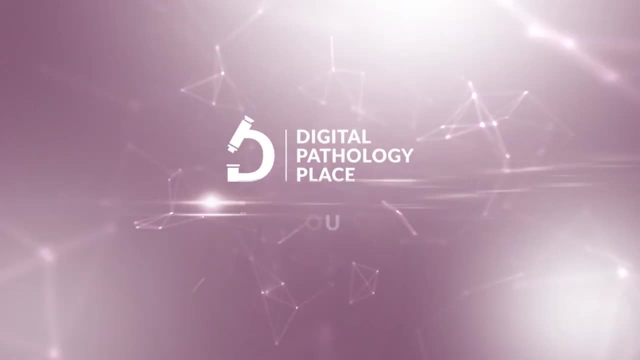 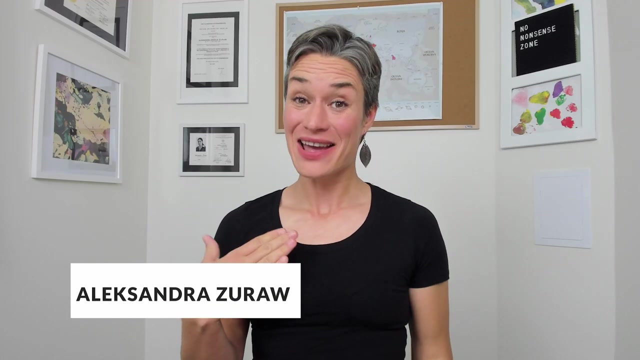 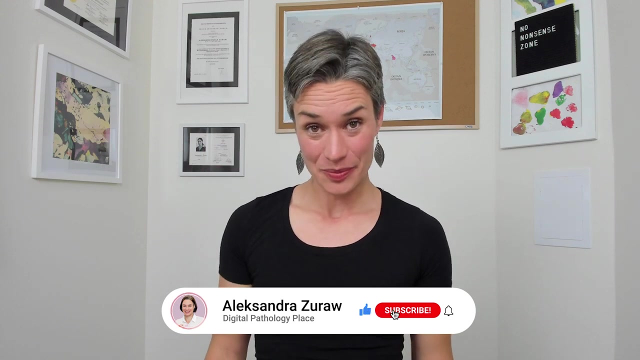 learn about in this video. Hi, I'm Aleksandra Zhurav and I'm here to help you do better digital pathology. So if you're interested in learning about digital pathology and tissue image analysis, this is your place. So click the bell below, subscribe and be notified every time I 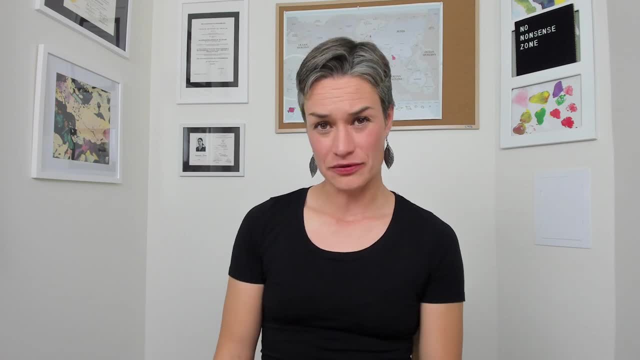 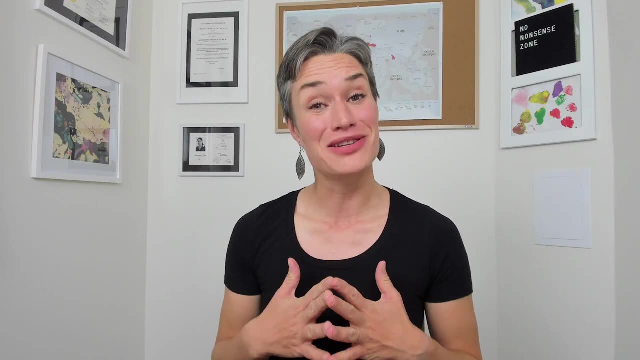 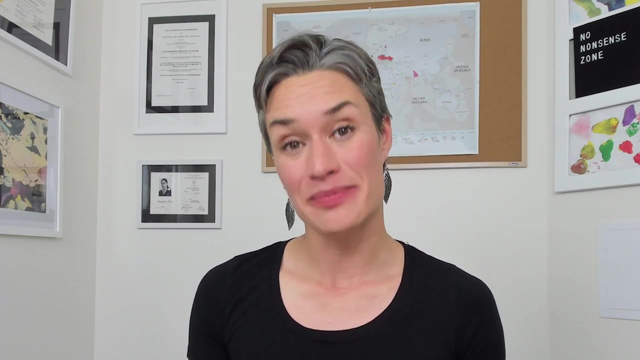 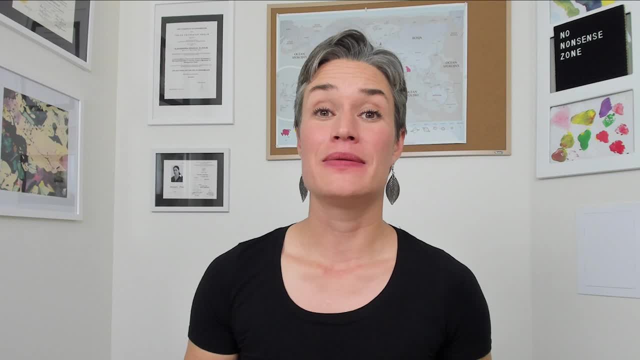 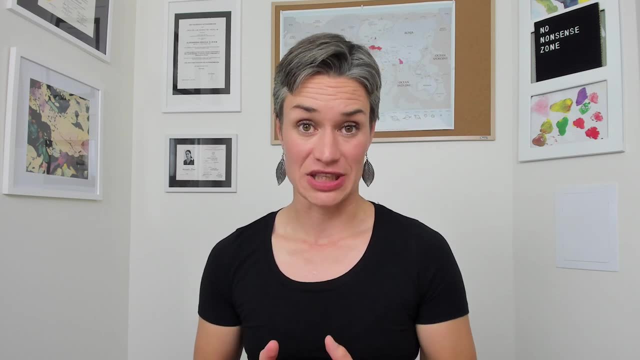 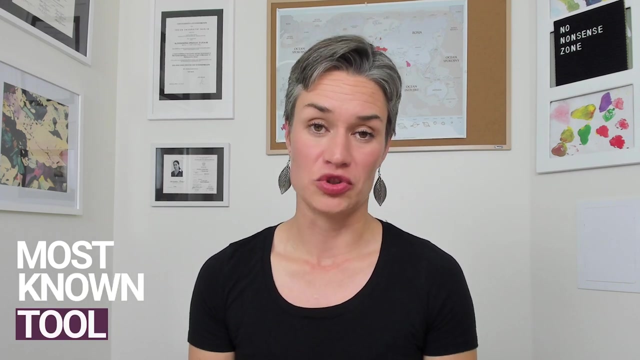 a software that allows you to do a lot of things. It's a Java based processing program developed in collaboration with National Health Institute and laboratory for optical and computational instrumentation, And this one is probably the most known in the whole bio image analysis community, not only pathology or tissue image analysis community. There are countless 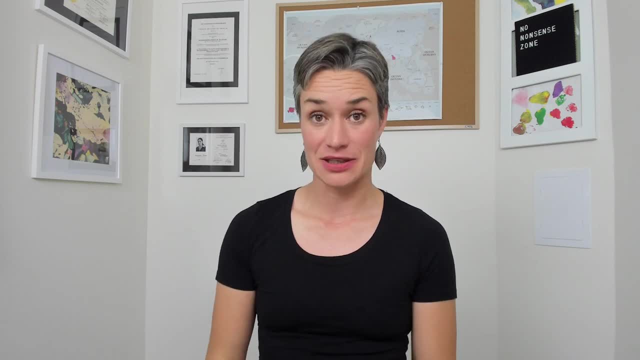 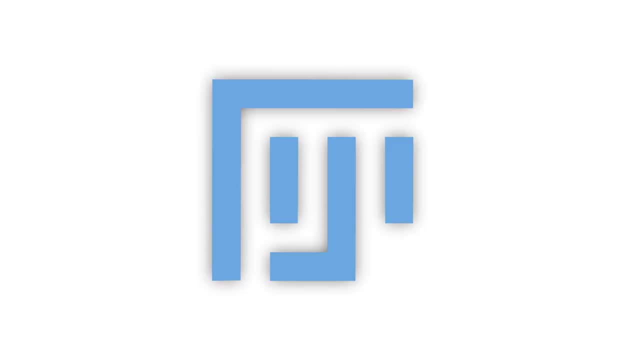 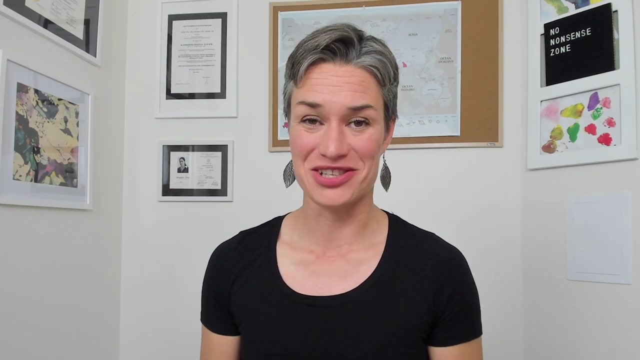 plugins for ImageJ and they cover different aspects of bio image analysis, And ImageJ is a mother program, so to say, of Fiji. Fiji is a distribution of ImageJ, basically a bundle of ready-to-use ImageJ plugins that you can use for image analysis, for tissue image analysis included. 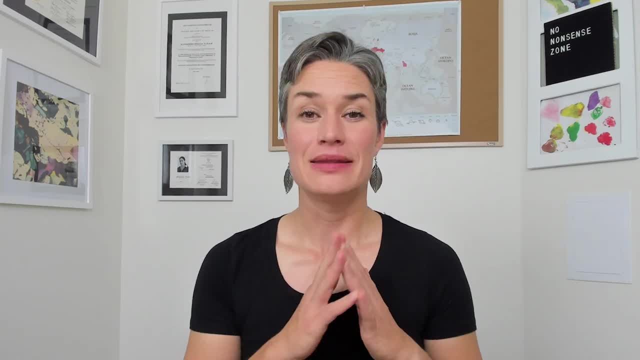 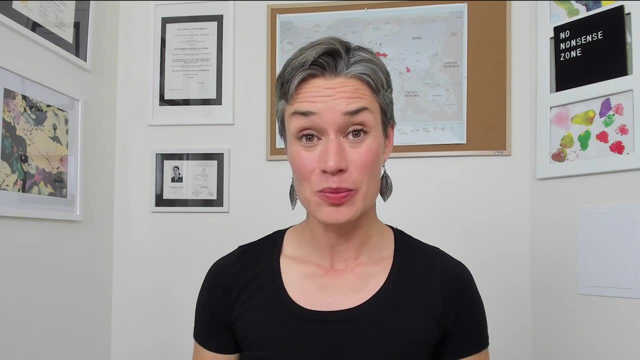 There is an ImageJ plugin that can handle whole slide images. The level of skill necessary here is basic. Researchers with basic computer skills can use it. but it is also cool for developers because they can develop plugins. So ImageJ is number one and I'm going to have a link in the 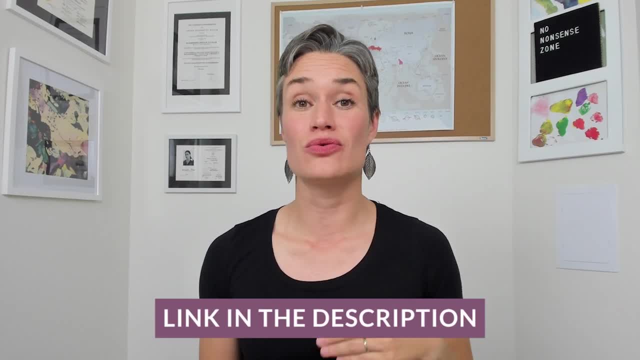 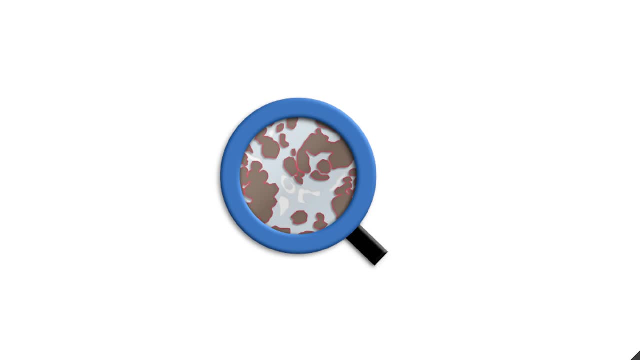 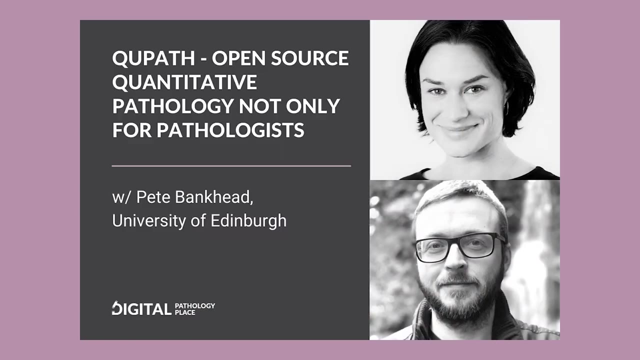 description to a PDF with all the links to where to download those images, where to find tutorials and how to navigate them. Number two is QPath. QPath, developed by Pete Bankett, who I was honored to interview as a podcast guest at some point, and I'm going to link to this podcast in the 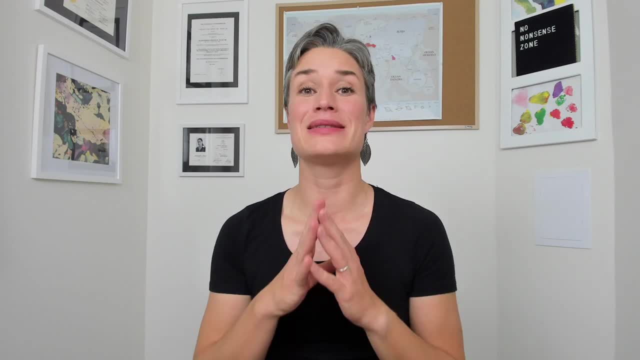 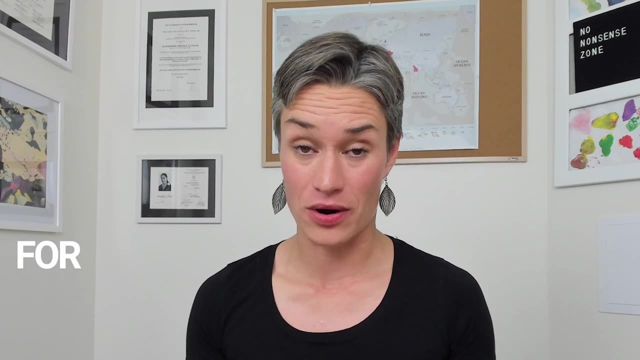 description below. It was just an audio podcast, but QPath is designed specifically for whole slide images- ImageJ. you can have a plugin that handles them. QPath is for whole slide images. QPath is designed specifically for whole slide images- ImageJ. you can have a plugin that. 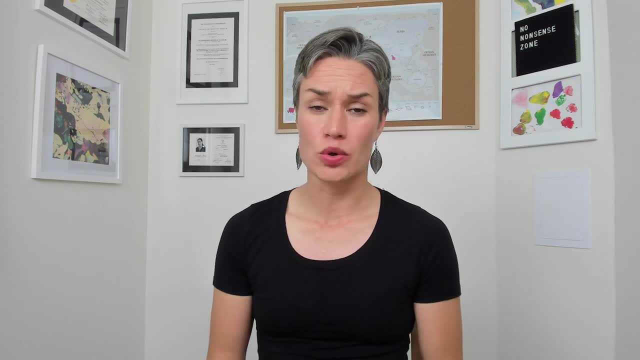 handles them. QPath is for whole slide images. QPath is designed specifically for whole slide images. In the first place it was developed for biomarker quantification, for immunohistochemistry quantification, But the scope is now a lot broader. 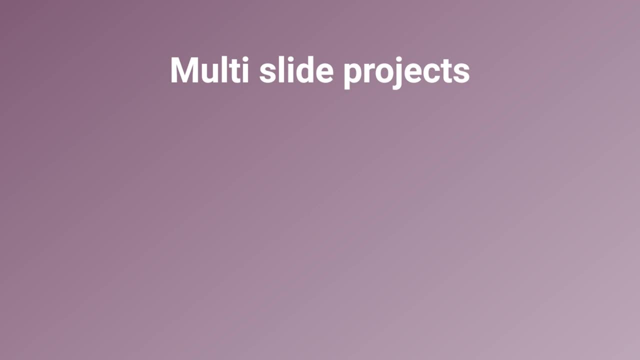 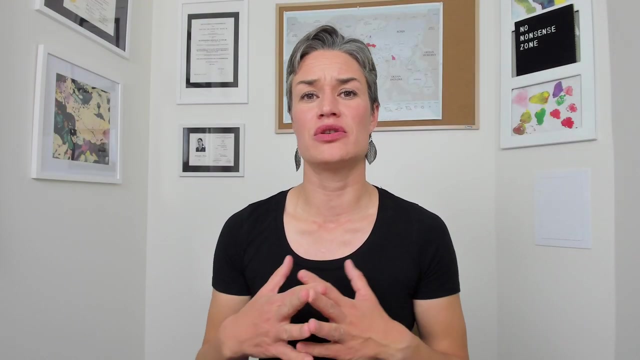 And in QPath you can create multi-slide projects. You can do stain estimation, You can do annotations like very sophisticated annotations, You can do cell quantification and all the different things that you would expect from a really high-end tissue image analysis software. 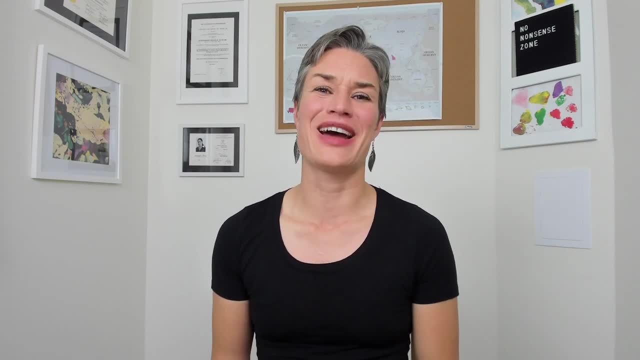 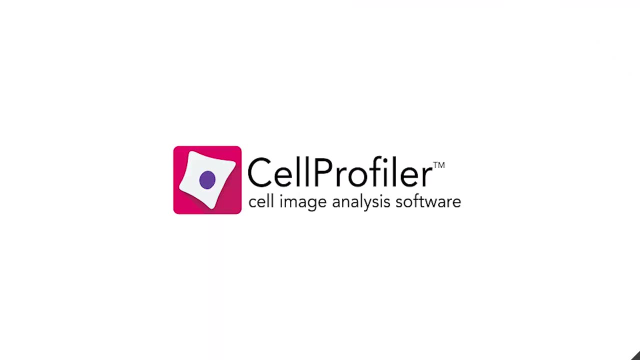 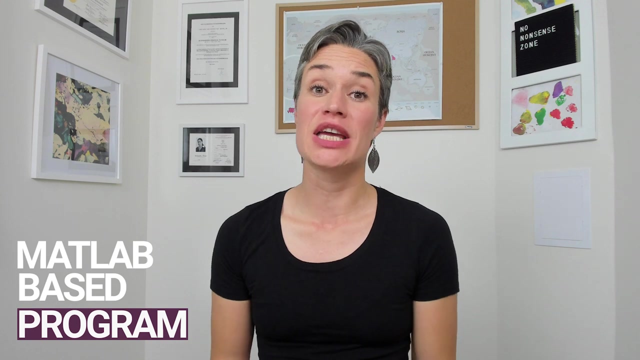 So congratulations to Pete, And there's a cool story behind it, So be sure to check in the podcast that is linked in the description. Number three on our list is Cell Profiler, developed at MIT and Harvard. This is a MATLAB-based program for batch processing cells in biology. 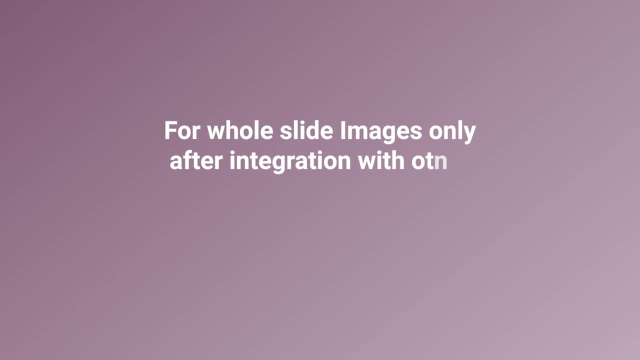 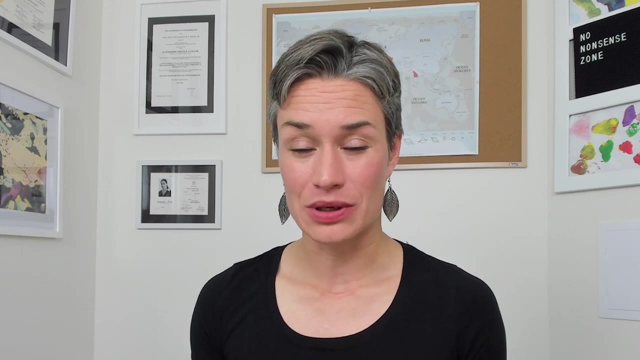 This one is good for biology and for cells, but it can only be used with whole-slide images after integration with other programs such as Orbit. Before we move to the next point on our list, all of those programs were developed in some kind of scientific way. 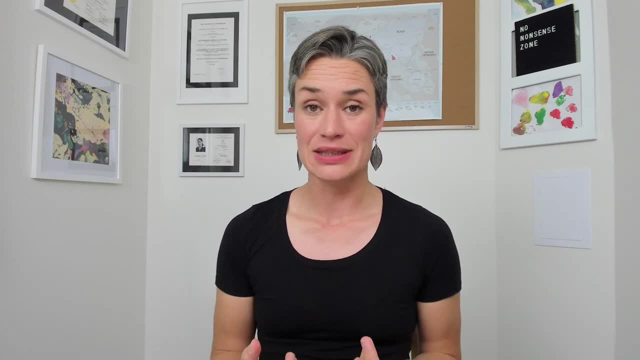 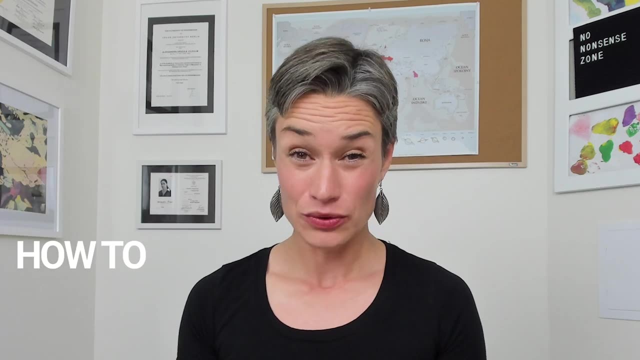 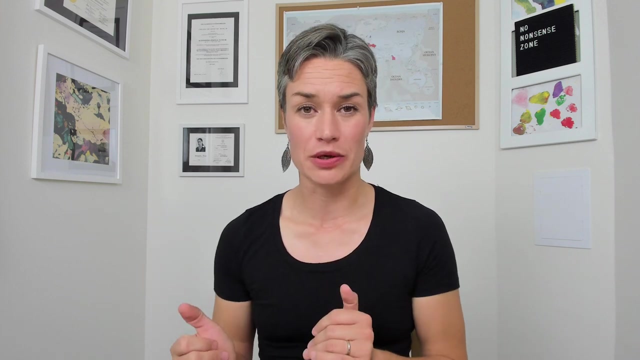 They're called scientific collaborations. So whenever you're using them for publication, be sure to cite them appropriately. And in the PDF there is going to be the links: how to cite them, how to cite each of those programs. So, even though Cell Profiler is not really for whole-slide images, you can find a workaround. 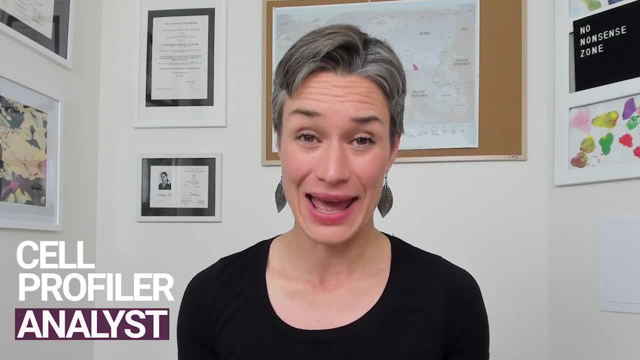 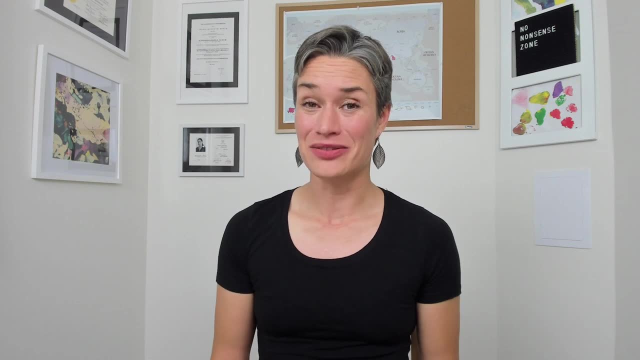 It comes with something cool that's called Cell Profiler Analyst. This is not really an image analysis software, but this is data analysis software. A couple of times I have already encountered not the tissue image analysis software, but the data analysis software. 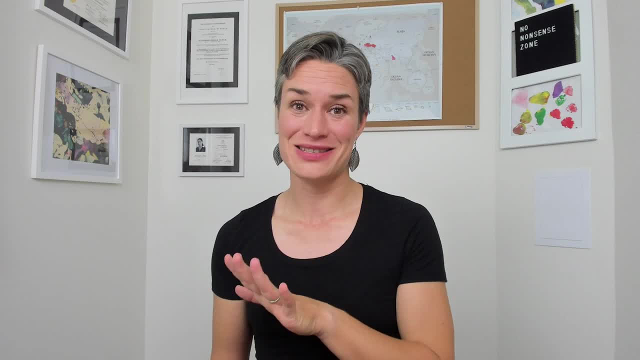 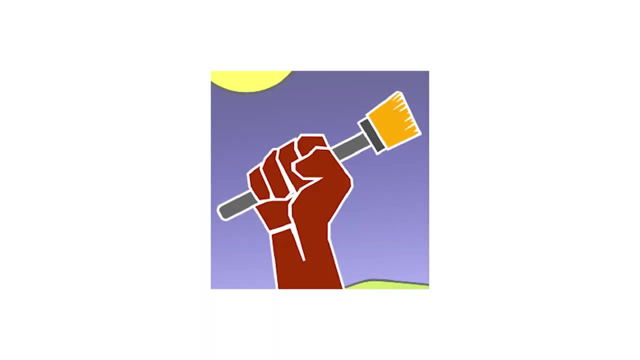 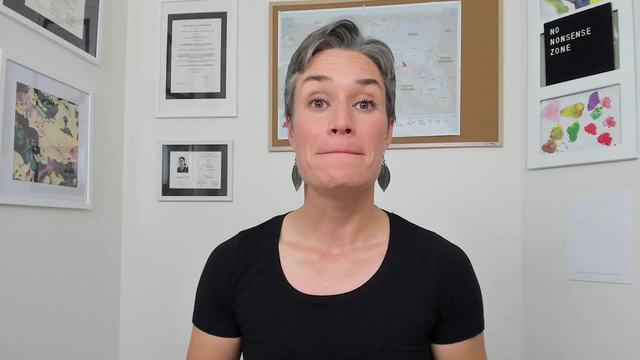 The data analysis process is difficult for me, but the analysis of data, So this has a specific program to analyze your data. Number four on the list is Elastic. This one allows users without expertise in image processing to perform cell quantification, meaning segmentation and classification of 2D, 3D and 4D images in a unified way. 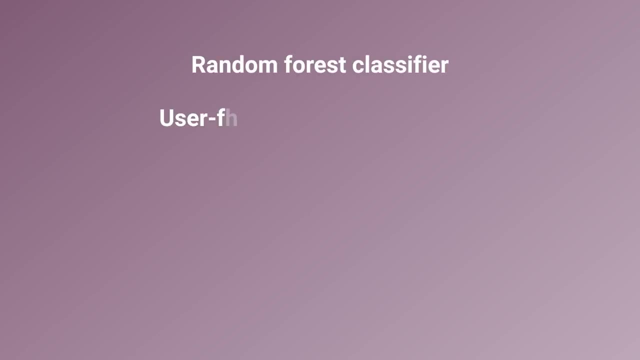 It includes the random forest classifier. It has a good graphic user interface. It enables the user to interactively refine segmentation because there is a real-life feedback. There's an option to integrate into Cell Profiler batch processing pipeline and developers can also design plugins. 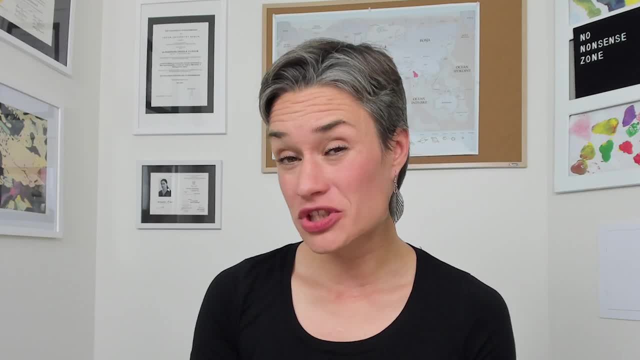 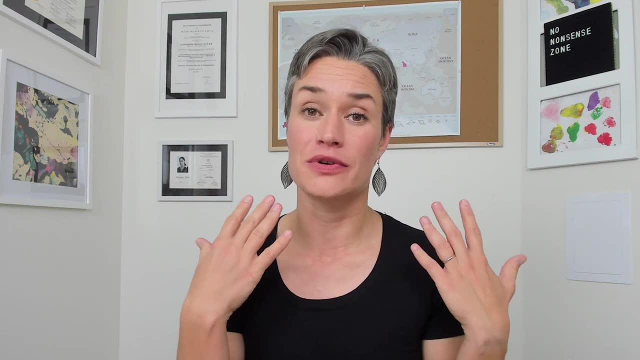 Sad story for those who want to do tissue image analysis. Unfortunately this one does not support whole-slide images, but high power fields of whole-slide images, so static images out of microscopic images can be analyzed. Too bad, because this has some cool features like uncertainty. 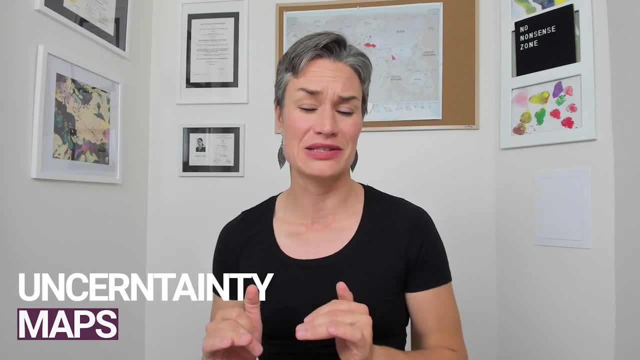 So static images out of microscopic images can be analyzed. Too bad, because this has some cool features like uncertainty. So static images out of microscopic images can be analyzed And it highlights where the model is the most uncertain. So that's kind of cutting edge features too bad. this one cannot be used for whole-slide image analysis. 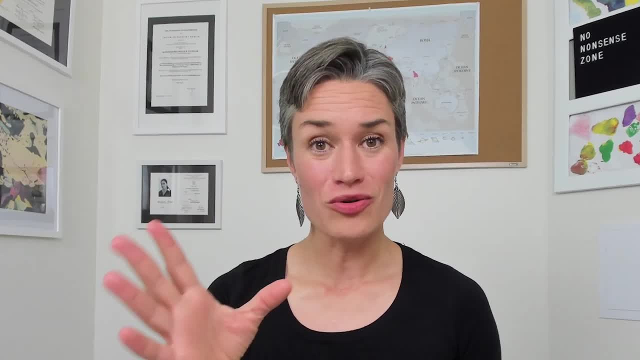 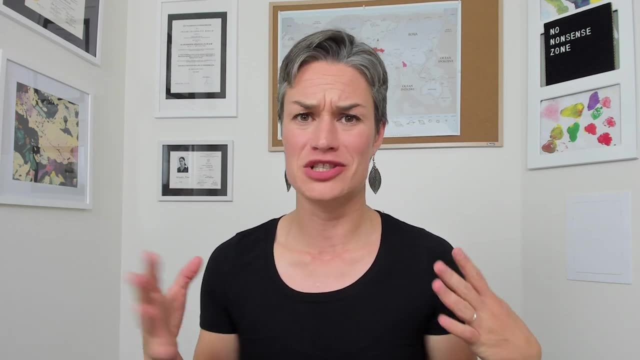 But even if it cannot be, the code can be used and can be used in future tools that are for whole-slide images. So all developers, digital pathology developers from throughout the world- this one has cool features. Check the code and maybe you can implement something in your software. 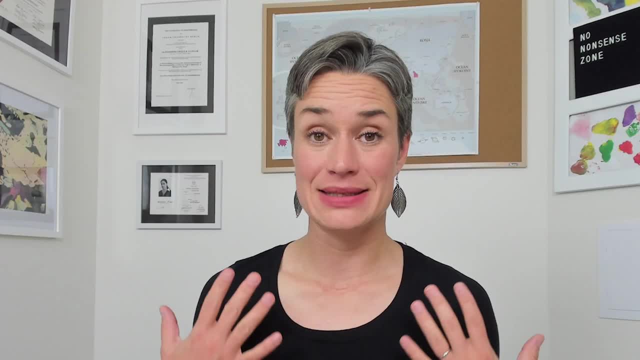 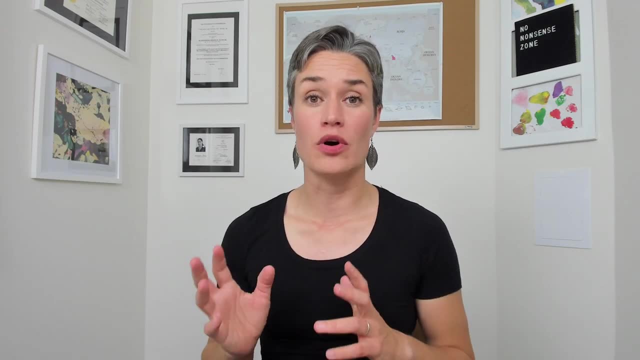 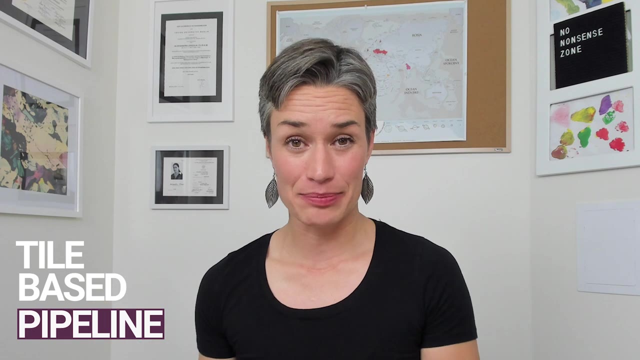 Number five is Orbit. Orbit is designed for quantifying very large images, including whole-slide images. It can load images from the local disk or it can connect to OMERO open microscopy environment, And processing of whole-slide images is due to the tile-based pipeline, as well as working on different resolutions of the image. 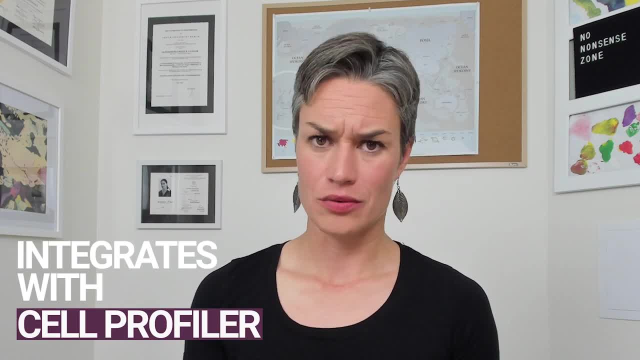 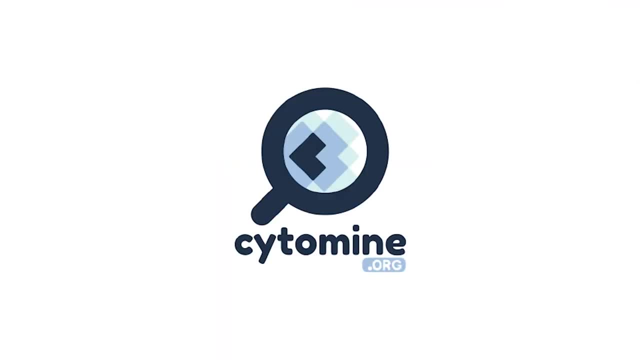 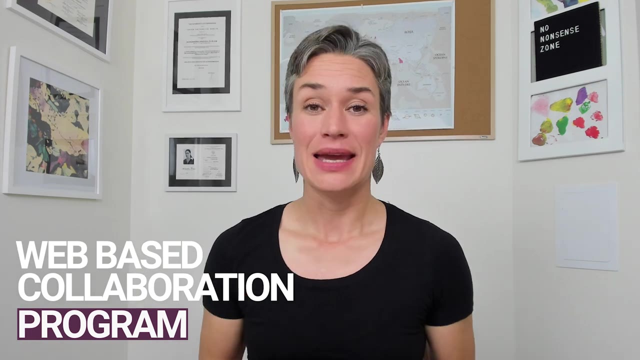 And Orbit also integrates with Cell Profiler. Well, well done, Cell Profiler people. you integrate with almost everything. Number six is Cytom. Cytomine is a web-based program that is very much focused on collaboration. It can be used by pathologists for annotations, by developers for developing models and deploying in Cytomine. 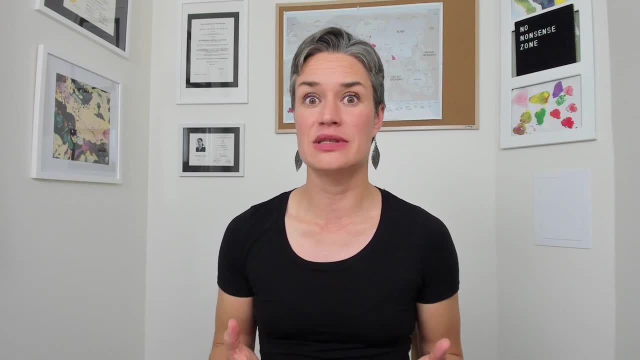 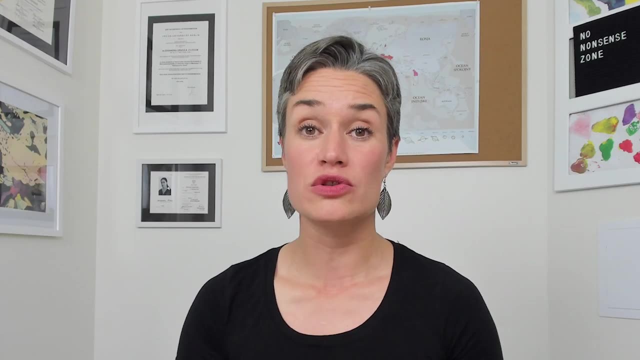 It also has the image management capabilities. It basically was designed for collaboration, for collaboration of everyone who is involved in tissue image analysis, So this one supports most of the whole-slide image formats. Something that's cool for me is that you can view multiple images next to each other. 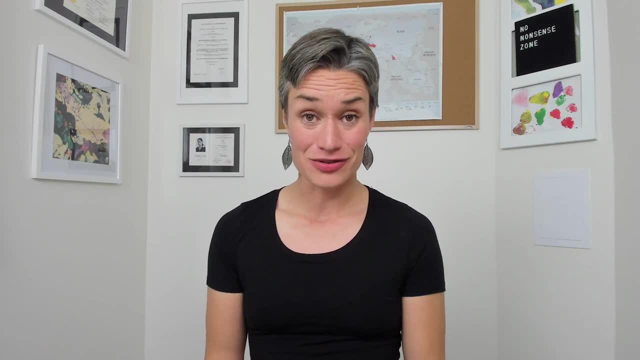 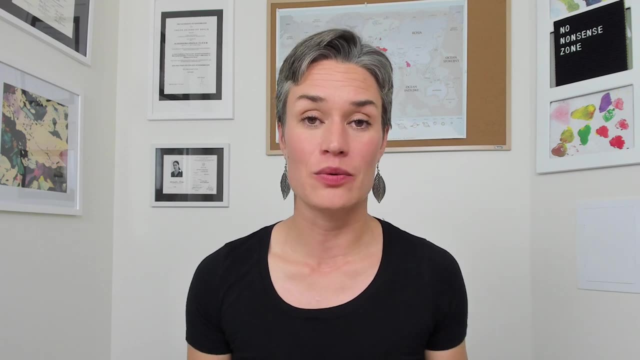 You can annotate. I'm a pathologist so obviously those pathology-centric features are going to be important for me. But the developers can basically develop locally in their development language and then deploy algorithms in Cytomine. And recently I talked to Gregoire Vick.